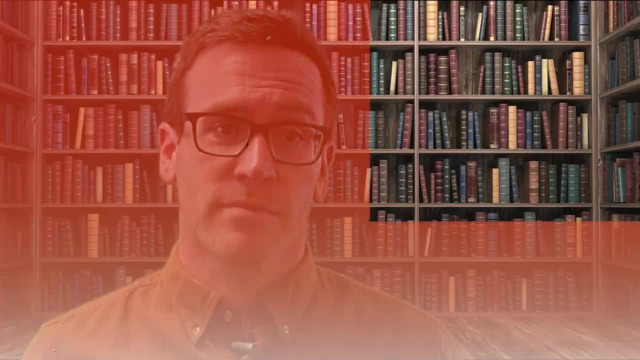 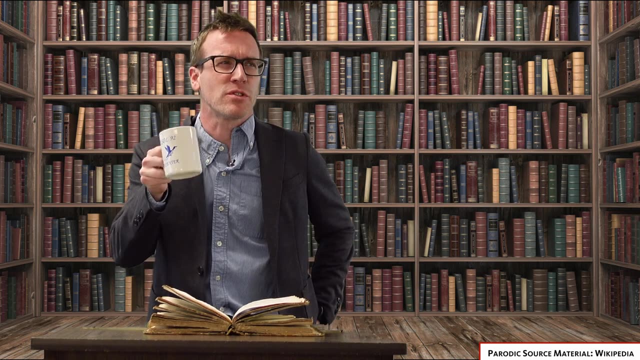 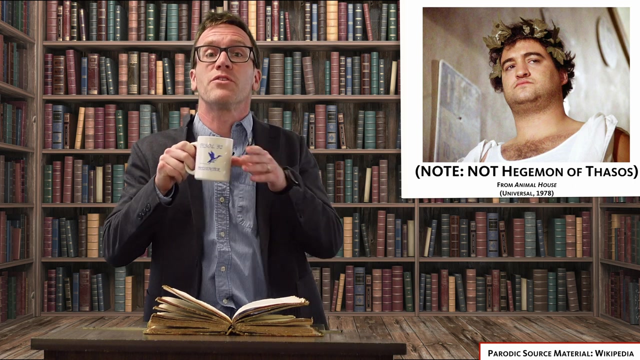 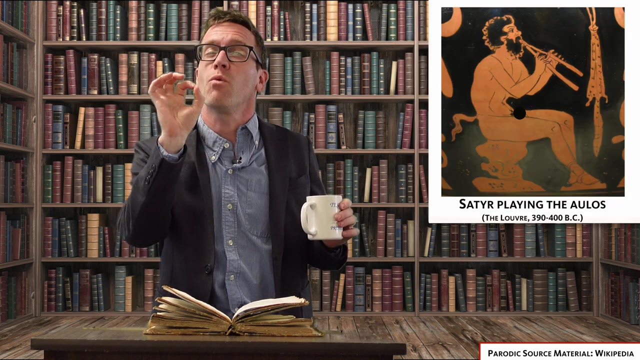 a book, a writing style or a real-life person. According to Aristotle in his Poetics, Chapter 2, Hegemon of Thesos was the inventor of parodies, though little of this playwright's works have survived until today. Aristotle claims he changed the wording in well-known poems in order to create: 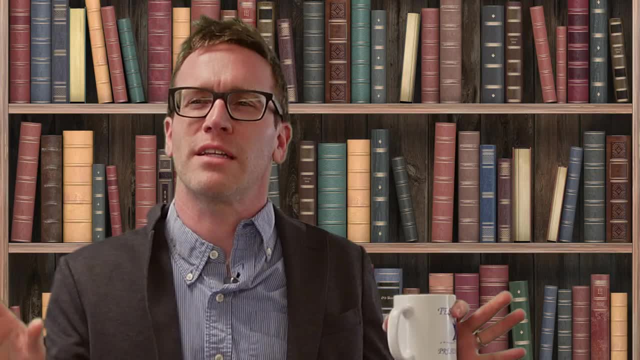 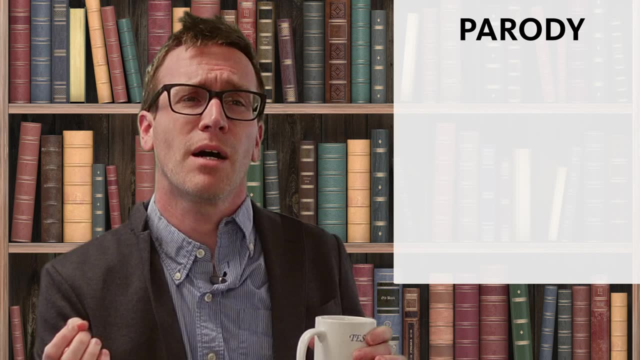 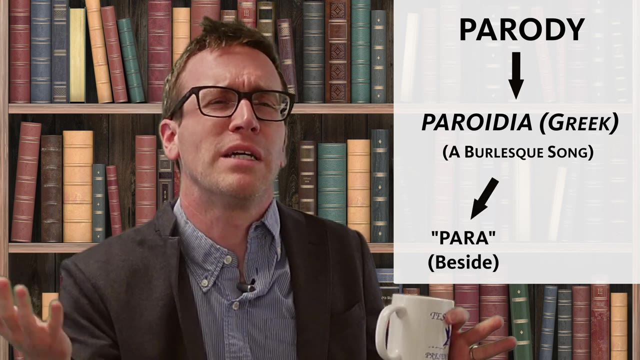 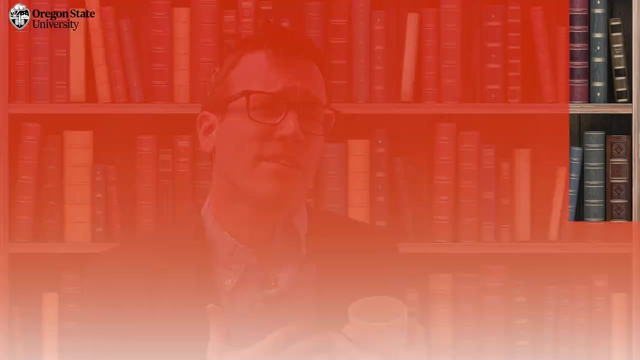 a humorous effect, thereby turning the sublime of the world into the ridiculous. The word parody itself comes from the Greek parodia, which means a burlesque song or poem. para, of course, meaning beside, and oid meaning song or ode, which are elaborate poems that the Greeks wanted us to write about. 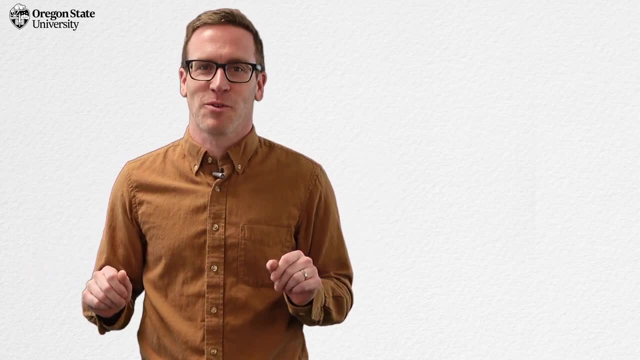 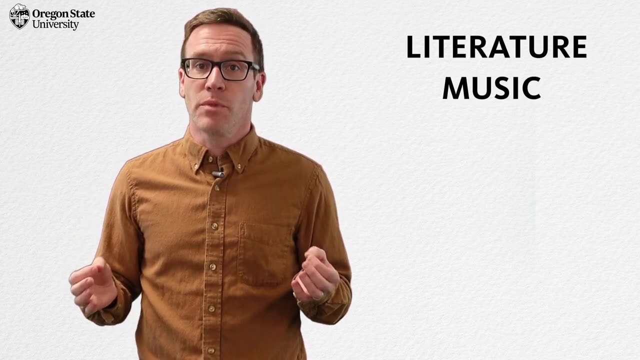 Uh sorry, there For a second I think I slipped into a parody of an English professor. Parody itself may be found in most any act of art or culture: literature, music, video games, movies, theater and more. Think of Weird Al, Most of his songs. 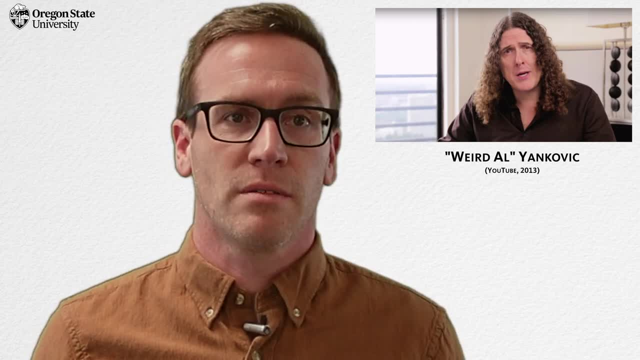 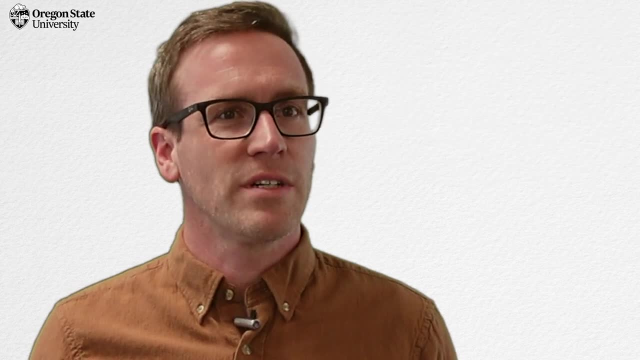 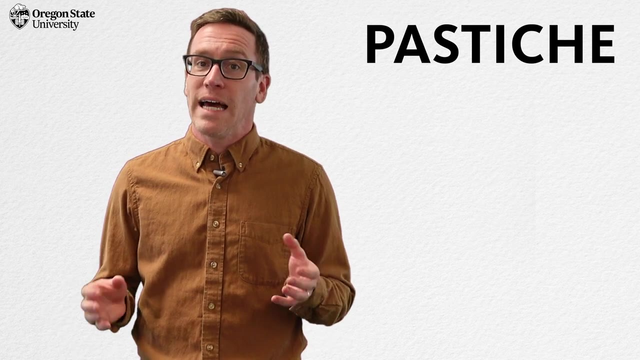 are parodies of something or someone in particular. Sometimes he makes fun of an artist and sometimes he makes fun of a song. One thing to note is that parody is distinct from both pastiche and satire. A pastiche is a work of art, and again it can be a form of literature, theater, film, etc. But what? 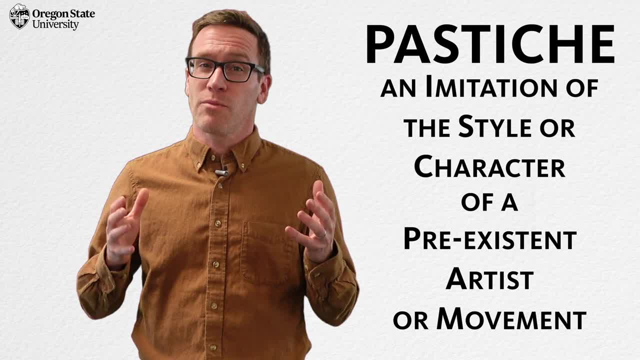 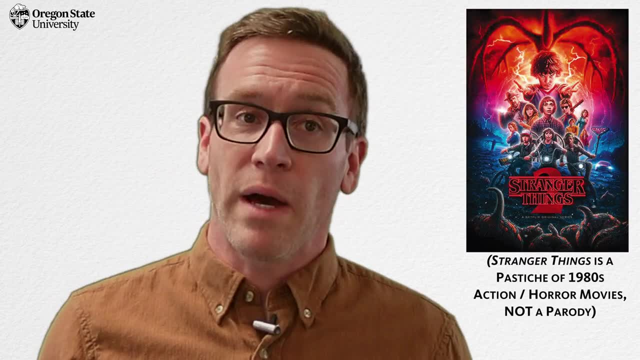 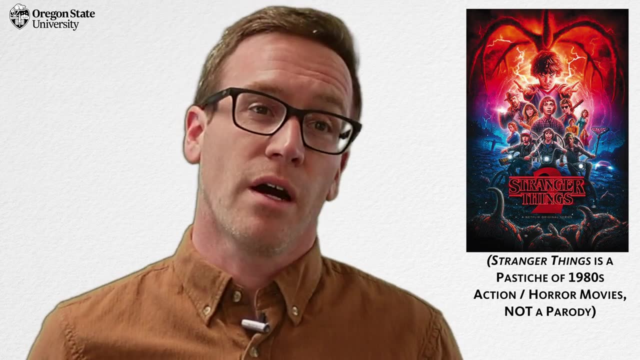 makes pastiche different is that authors of pastiche attempt to imitate the style or character of other artists, Sometimes not successfully. Creators of pastiche try to pay homage to an original work and can reproduce features of that art in a way that signals to their audience that 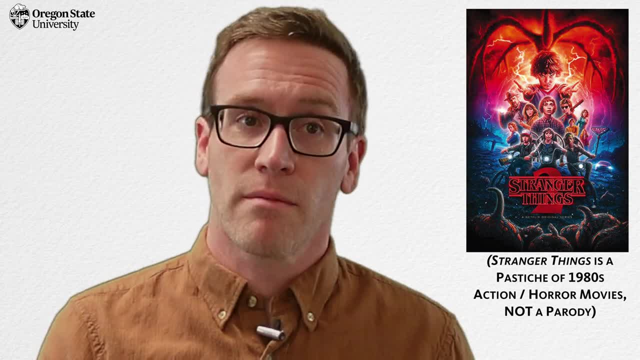 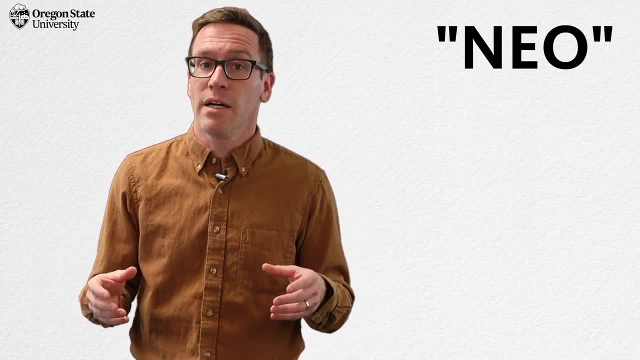 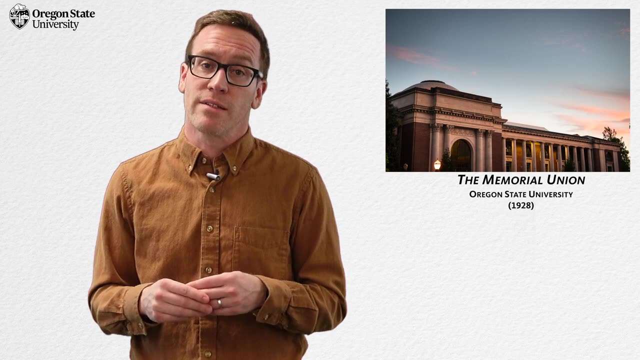 they are trying to imitate, though not directly copy, that earlier work. In architecture the word neo is often used to suggest that a particular style is done in homage, so neoclassical architecture is often a pastiche of Greek and Roman buildings and styles. 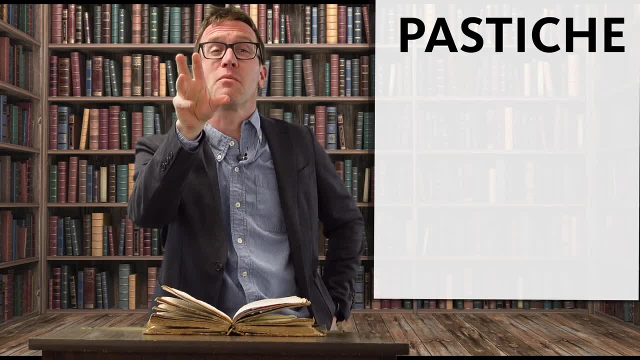 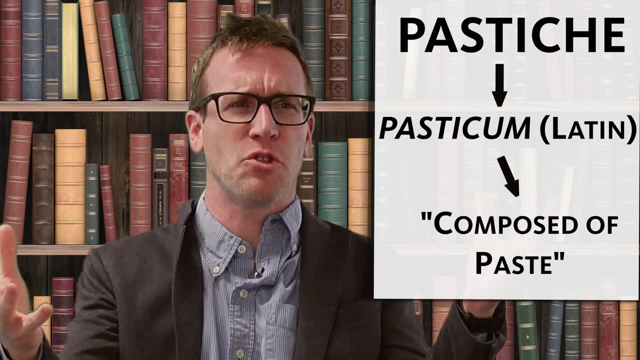 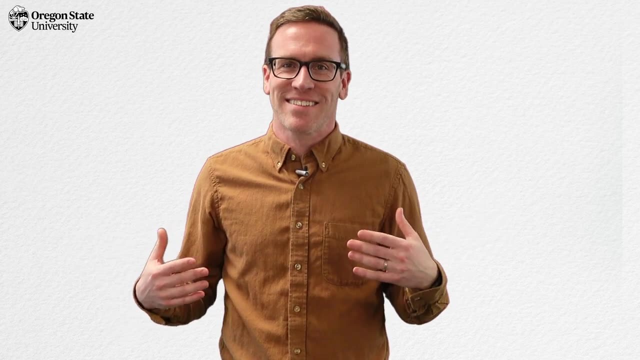 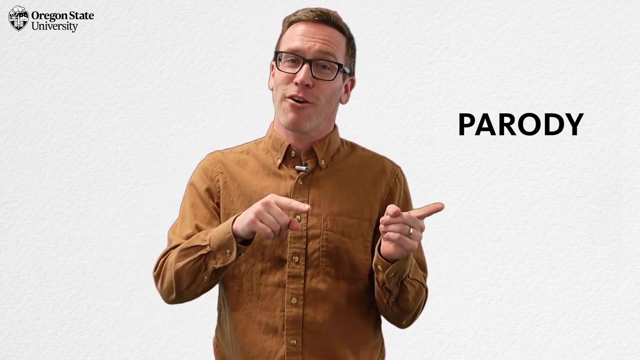 Pastiche comes from the Latin pasticum, which means composed of paste and is related to pate and pasta, among other words. Whoops, slipped back again into that English professor. Where was I? Oh yeah, I was just about to mention the difference between parody and satire. The difference is that 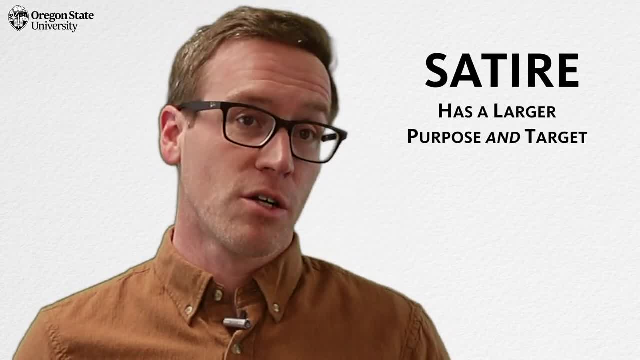 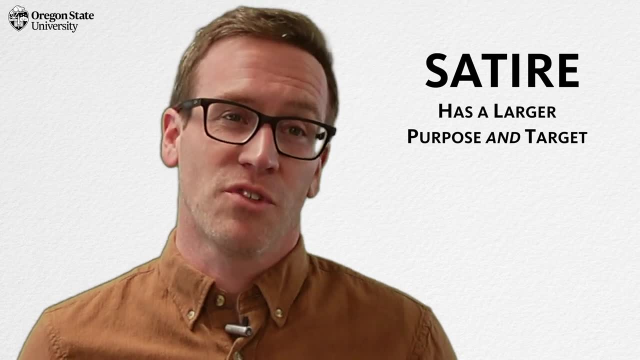 satire, while also supposed to be funny, often has a larger purpose. Both parody and satire will frequently make fun of something, but satire doesn't target a specific author or work. Satires will usually make fun of something, but satire doesn't target a specific author or work. 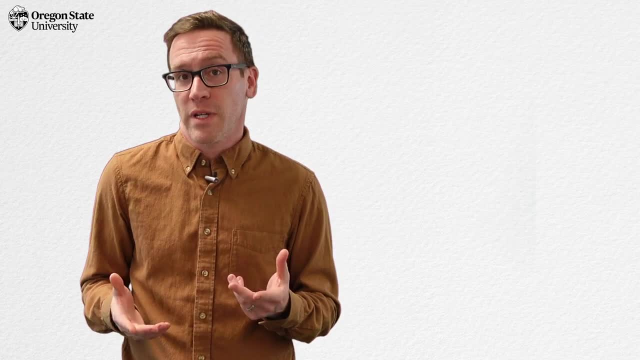 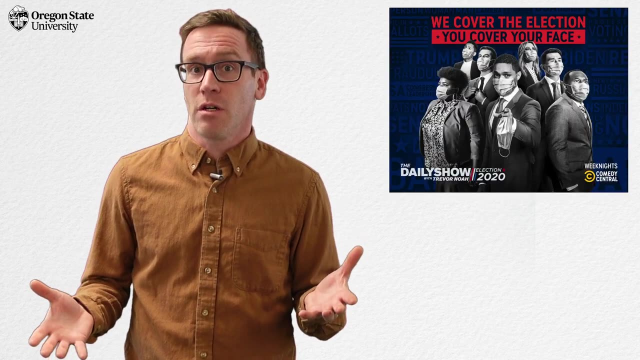 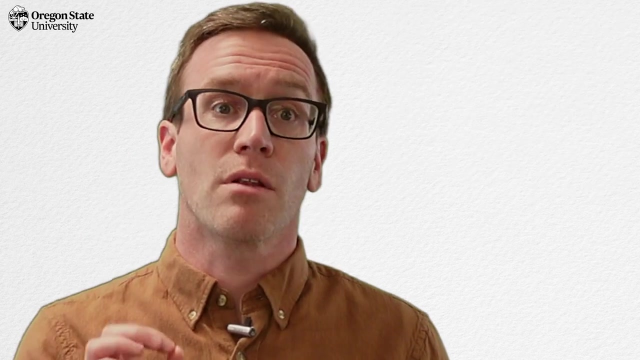 Satire can make fun of a genre, a cultural belief or a social movement and, in doing so, hope to critique society more generally. For example, The Daily Show uses loads of satire in its stories and most often critiques cultural issues more generally. And there are lots more. 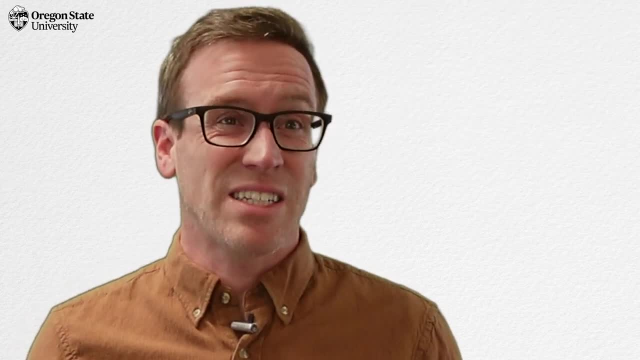 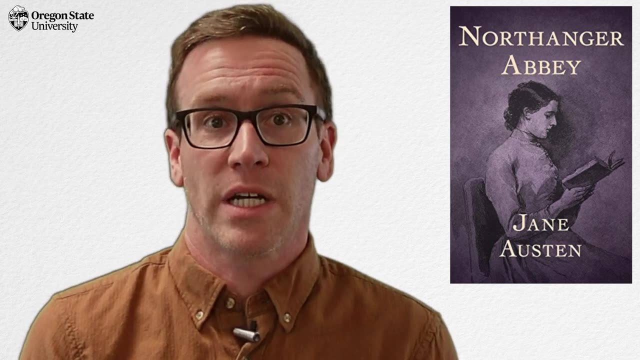 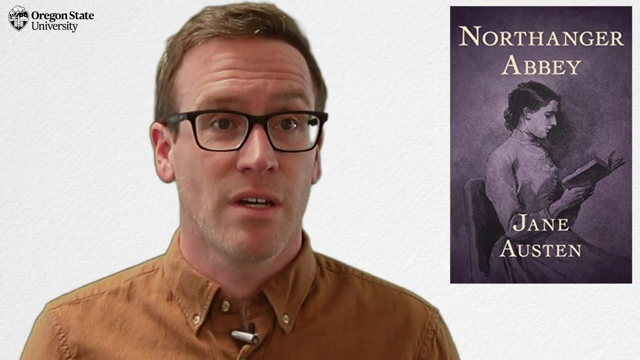 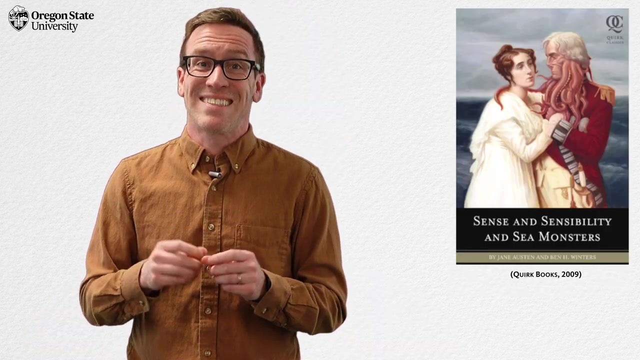 examples, some of which engage both parody and satire at once. Jane Austen's Northanger Abbey is a satire of middle-class appreciation of gothic knowledge And a critique of male-dominated politics and masculine standards of literary taste, But also a parody of Anne Radcliffe's The Mysteries of Udolpho Ben H Winter's Sense. 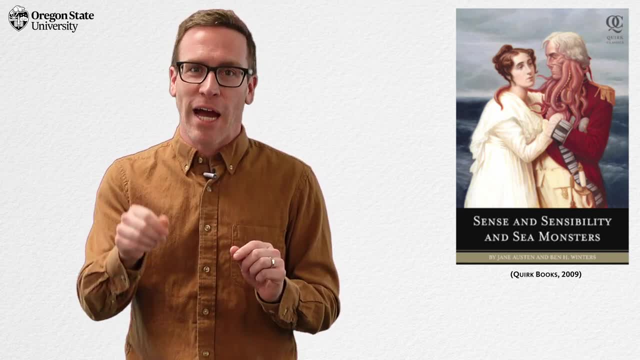 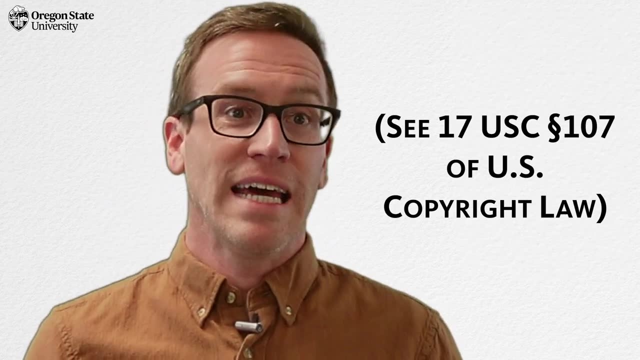 and Sensibility, and Sea Monsters, on the other hand, is a parody of Sense and Sensibility. Often, parody is a good defense against copyright infringement, at least in the US, because while parodies can copy some of the idea of an original work of art, 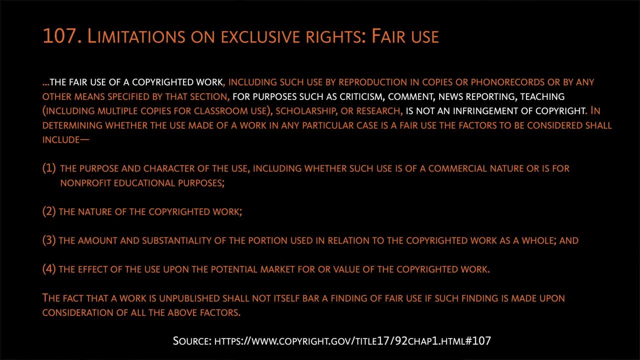 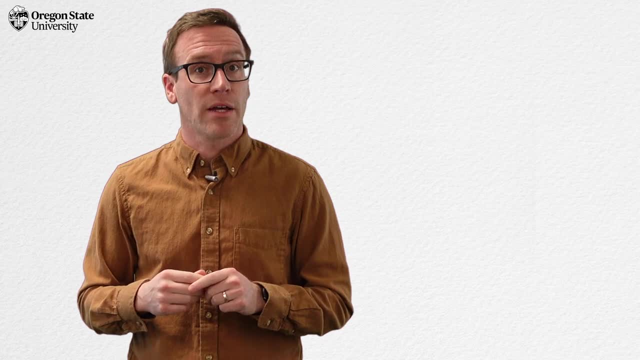 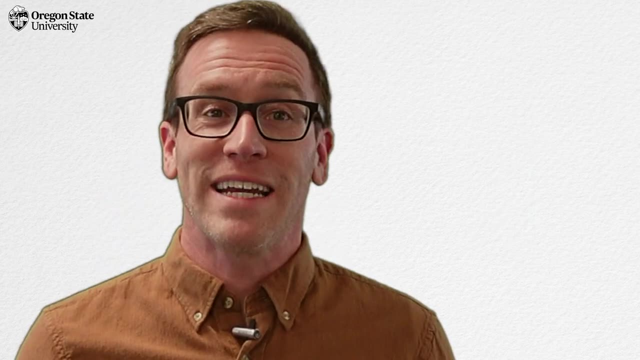 they also, crucially, comment upon that same work, thus transforming it and making something new. Parodies can also be tools that marginalized or oppressed groups can use to selectively appropriate or imitate aspects of other cultures. A great example of these elements is Alice Randall's novel The Wind Done Gone, which 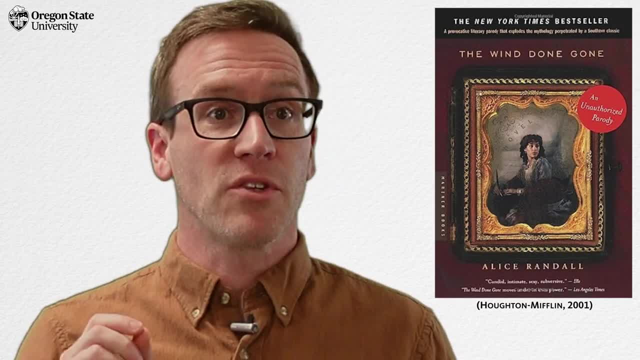 is a parody of Margaret Mitchell's Gone With the Wind, but told from the perspective of an enslaved person named Sonara, who lived for six months in the US and who also studied the modern world. The novel becomes a direct asset to the text, But of course, an introduction to the 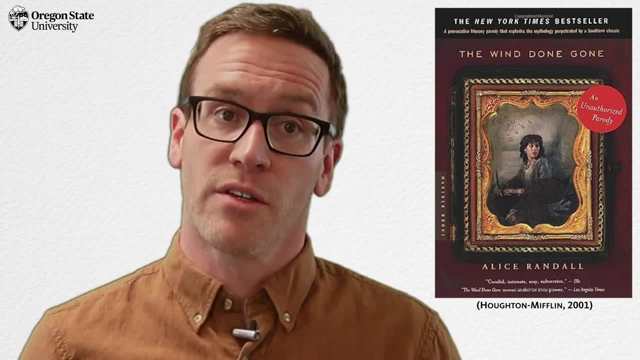 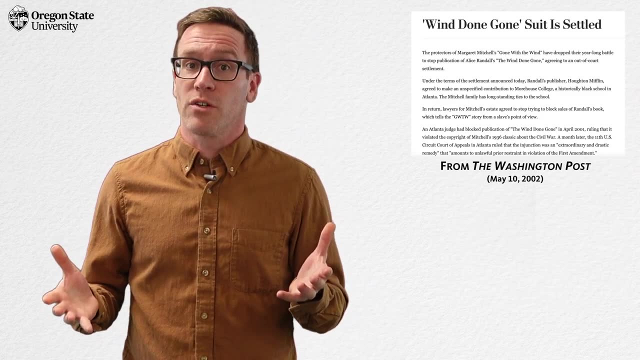 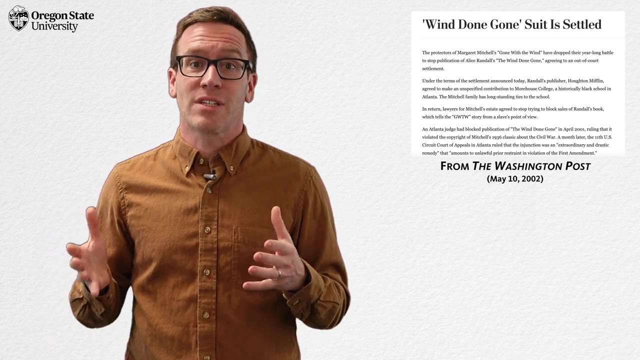 who has been recently freed, instead of Scarlett O'Hara, the southern white woman and part of the slave-owning family in the novel. The estate of Margaret Mitchell sued Alice Randall and her publishing company for copyright violation. The case was settled, but The Wind Done Gone is clearly.